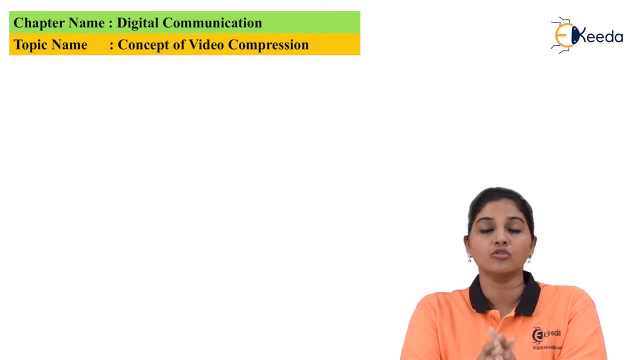 requires more space. so to avoid this and to utilize the available bandwidth and to utilize the available space more effectively, it is very much important to perform compression on such files. so the method of compression of video is called as video compression, or we can say a video compression is a method. 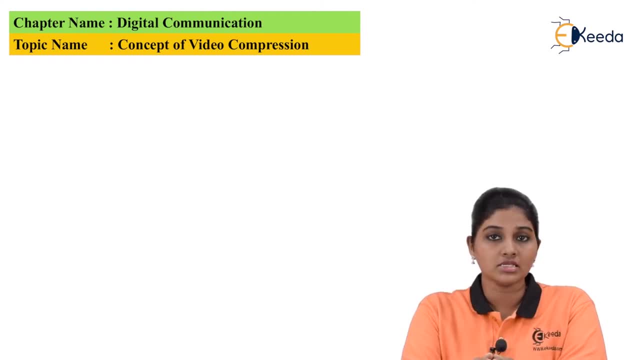 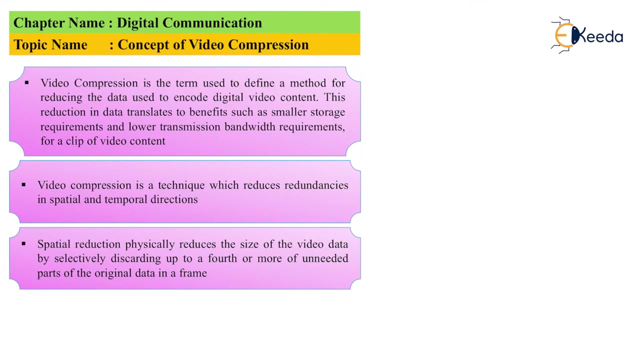 which is used to reproduce the file, which is having small size, and we can store that file onto the storage in by using a small space. so now let's see what do you mean actually by video compression. so basically, the video compression is a term used to define a method for 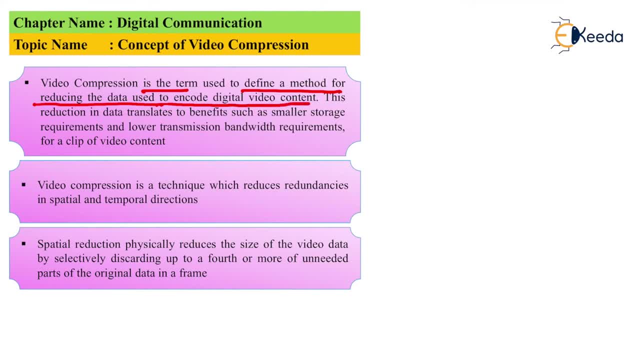 reducing the data which is to be get encoded digital video content. this reduction of data translates the benefits such as smaller storage requirement and lower transmission bandwidth requirement for a clip of video content. so whenever we want to reduce the file, whenever we want to use a space for storing more number of files, then we can perform a method or a technique which 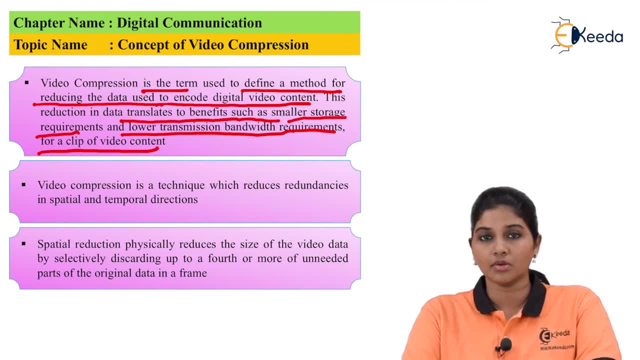 is called as video compression. so the two basic advantages provided by video compression is nothing, but it uses a lower bandwidth for the transmission and it provides more space for storing more data, more files, onto the disk. now it basically reduces the redundancy in the spital and temporal. 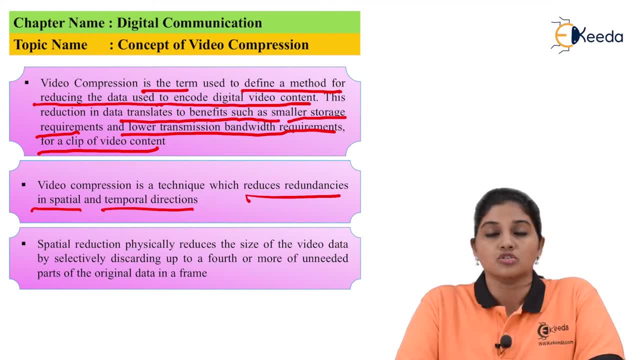 direction. so redundancy is basically stands for repetition. so if we delete the repeated image or if we delete the replications of the pictures, then it is possible to reduce the bandwidth of the signal or it is possible to reduce the size of the file. so it basically uses a technique. 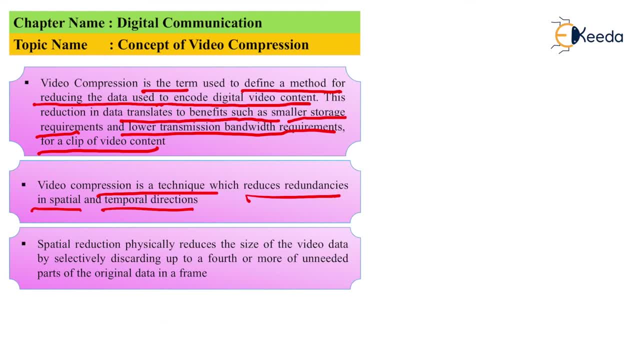 which reduces the redundancy in spital and temporal direction. now let's see what do you mean by spital and temporal direction in spital reduction: physical reduction in size of video data by separately discarding up to fourth or more unneeded parts of the original data frame. so 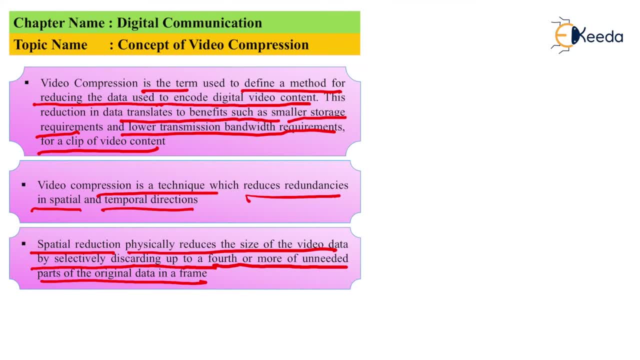 basically, here the actual separation and actual reduction of the file size takes place, where the signals which are repeated in nature, where the signals which are replica of the other signals are get deleted and they are get discarded up to fourth or four or more, which the label uses to select samples, so so that we can. 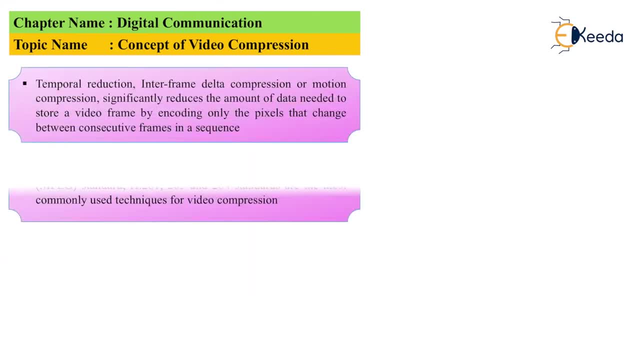 see the actual separation of the schwier has. ok, now don't you care about the expressive fire occupancy of the using differenceing. really important and in order to solve our problem are: and the media in which wasn'tall that the image and getting teste. this is for the data context of it to get understood by the material. and making sure that the data- handsome it will be buttoned and now the two cells by are anytime. but he does an區 what we do not have the Mexico from. but it would have been an area from C nation and the current number. they already have the amount of Savior possible. so it is now the future of the, as this would be a. 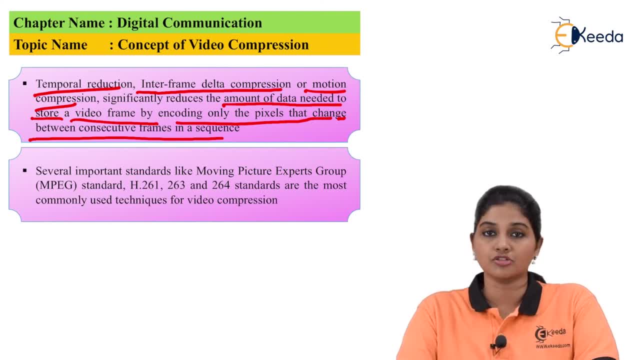 postage Texas. when we get here on the floats in this particular shape it need also in the consecutive frame of sequence, then it is possible to reduce the file size and the temporal reduction is also called as inter frame Delta conversion or inter frame Delta compression, or is it is also called as motion compression. 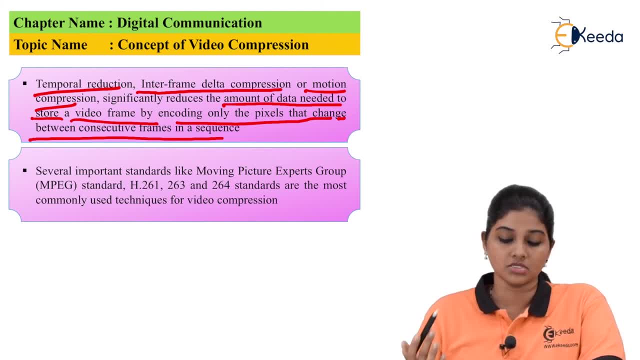 so these are the various names, but it uses the same technique. that means it encodes only the pixels which changes between the consecutive frame in a sequence. so there are various methods that can be used for compression of the video, and these are nothing but moving picture expert group, that is, MPEG. 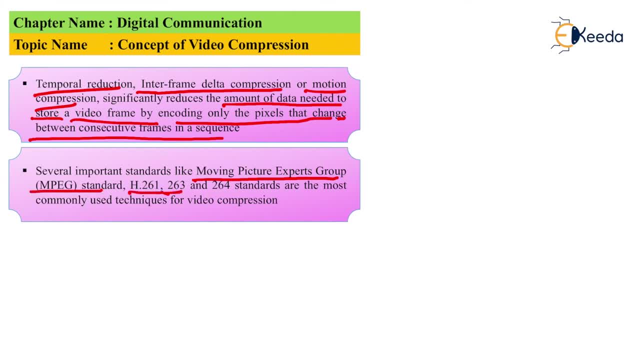 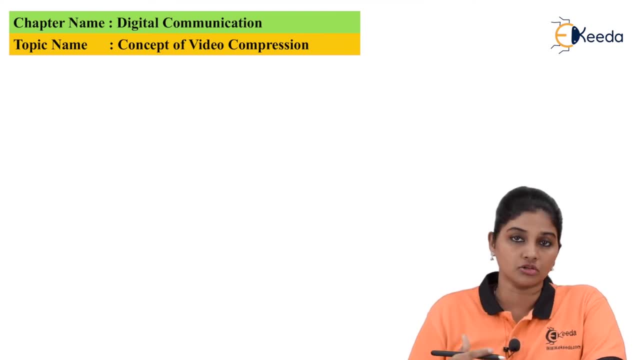 standard, then H 261, 63, 64 standards are most commonly used for video compression. now the three basic standards or the three basic methods which are used for video compression are: the first one is H 264. it basically most commonly used method and most widely used method. now, in this method, a small groups of images: 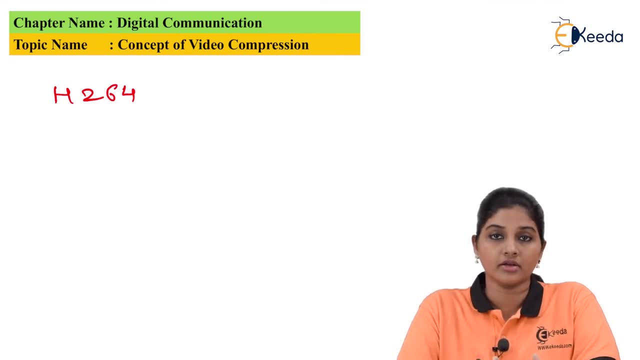 are get created in this a small group of images are they created and it use. it removes the replica so that those file size. it get compressed and the file size become really reduced to a lower value. the second type of method that is used for video compression is nothing but. 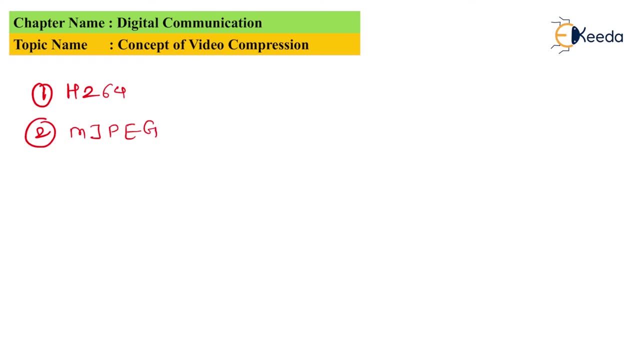 the second method is nothing but mjpg. it is also called as motion jpg because in this the individual image is considered as a frame and therefore it is called a as motion jpg. now the third method that is used for the video compression is mpg4. now this is considered as the oldest method and it is get commonly replaced by the first.